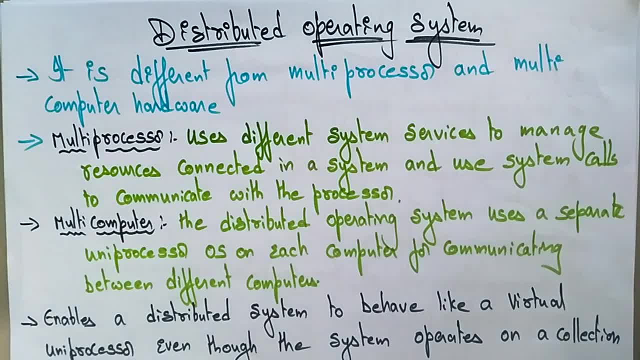 operating system. you are thinking that it may be it having a multi processors. Each system is capable of having the multi processor or it is a multi computer hardware. but it is not Okay. the multi processor is different, multi computer is different and the distributed is. 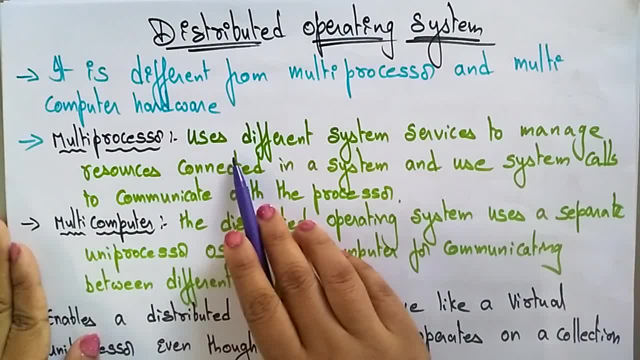 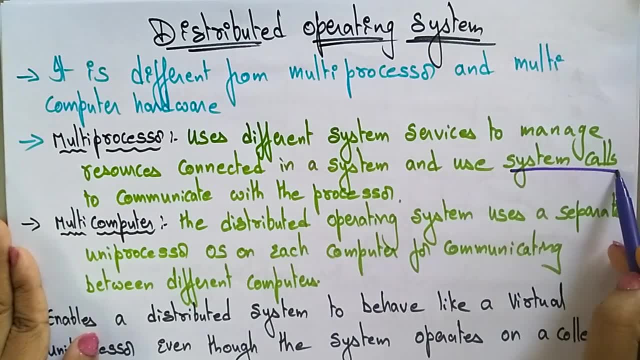 different. Then what is a multi processor? The multi processor uses different system services to manage resource connected in a system and use the system calls to communicate with the processor. This is a multi processor means here the user uses different system services will be using 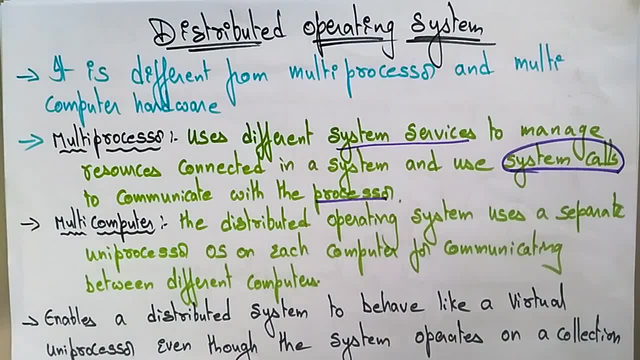 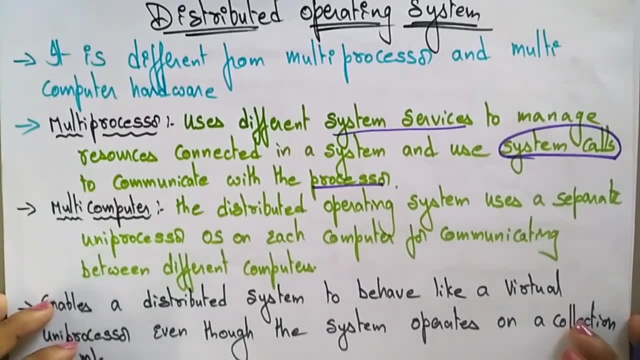 So that is why we are calling it as a multi processor. It is going to manage resource connected in a system By using the system calls with the processor. Then, whatever the multi computer, The multi computer, the distributed operating system, uses a separate uniprocessor operating system. 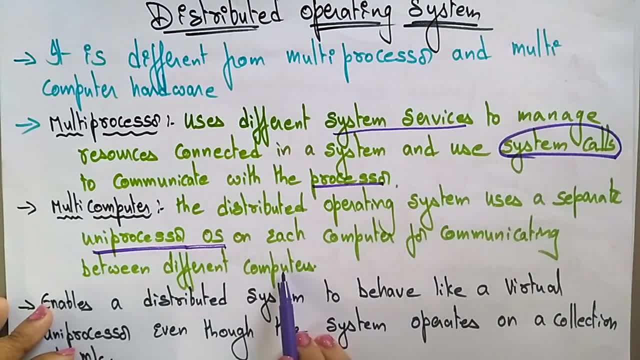 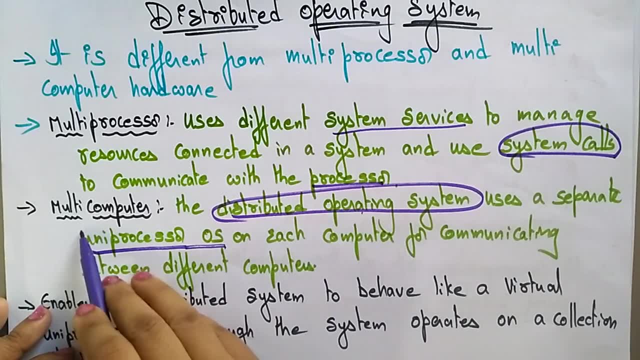 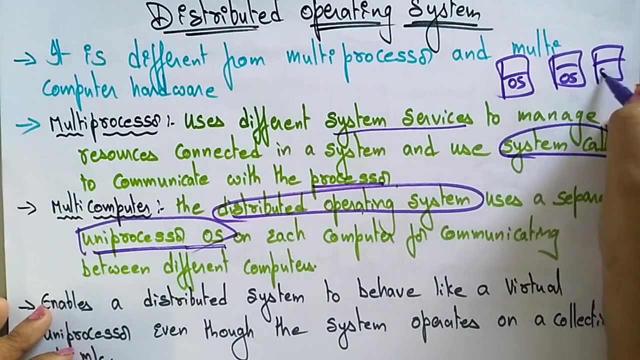 on each computer for communicating between different computers. So if you are using the distributed operating system, the distributed operating system uses a separate uniprocessor. operating system means each machine is having their own operating system. This you call it as a uni operating system. 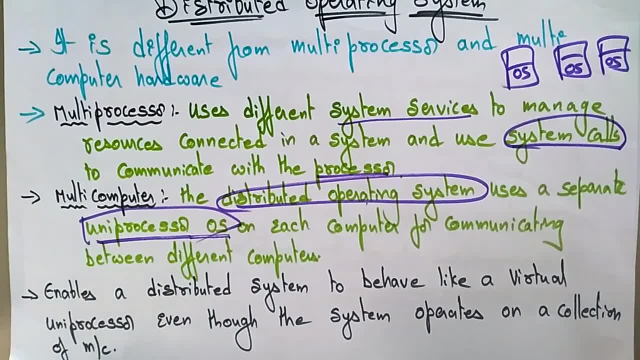 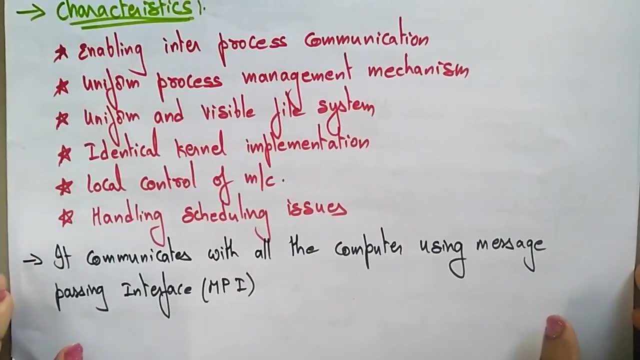 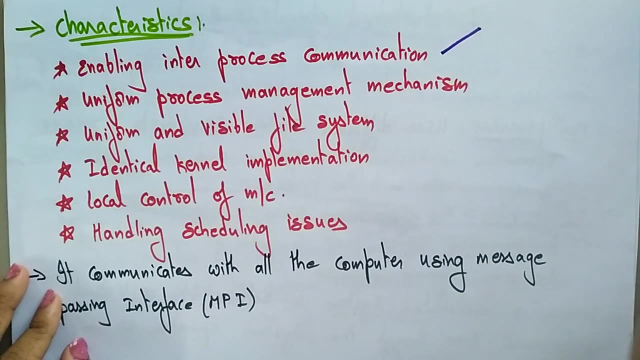 So it enables the distributed operating, enables a distributed system to behave like a virtual uni processor, even though the system operates on a collection of machines. Now let's see what are the characteristics of using this distributed operating system. it enabling the inter-process communication. The distributed operating system is enabling 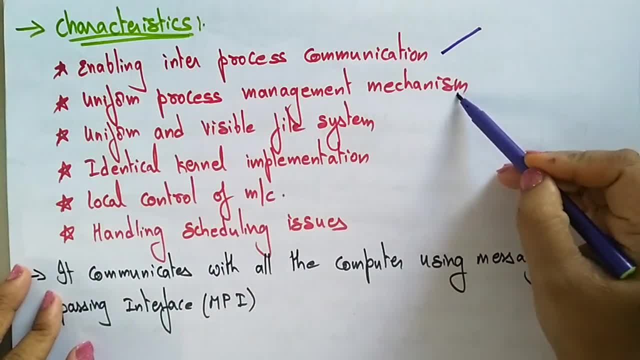 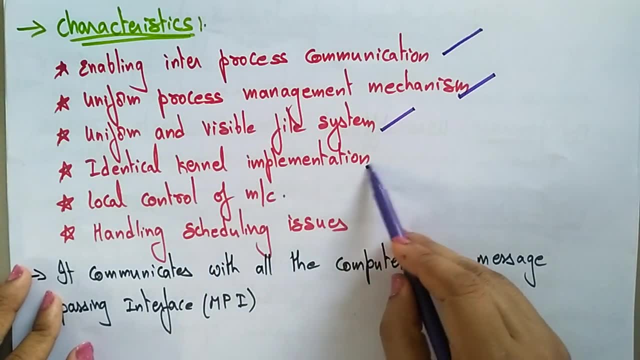 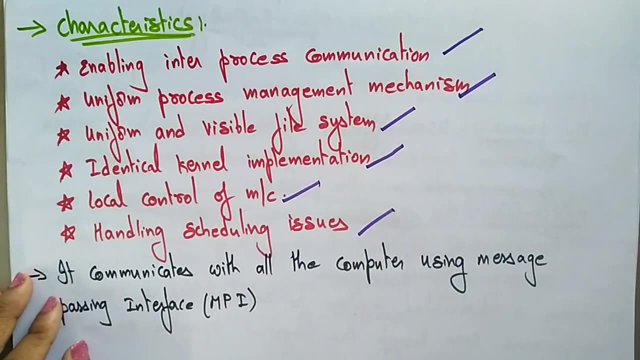 the inter process communication, uniform process management, maintain customer balance. Эdry mechanism is available, Uniform and visible file systems are there, Identical kernel implementation is there, Local control of machines and handling scheduling issues. So these are all the characteristics of the distributed operating system, And also it communicates with all the 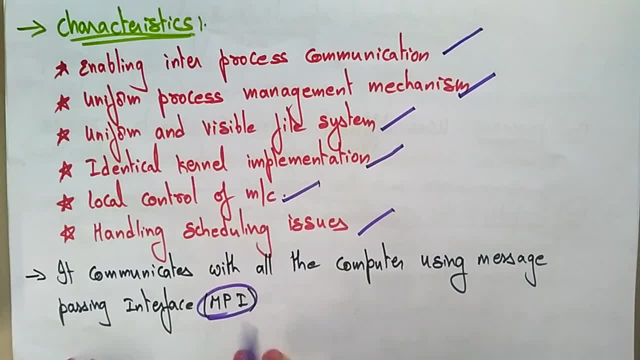 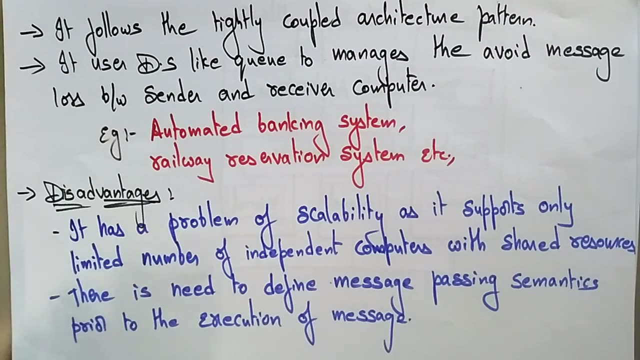 computers using one message, that is, MPI message passing interface. With the help of the message passing interface, the distributed operating system is going to communicate with all the computers And it also follows the tightly coupled architecture pattern. So, whereas the network operating system is a loosely coupled, follows a loosely coupled architecture pattern, but the